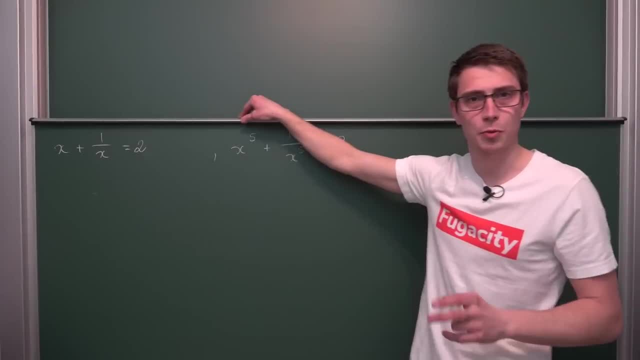 More information at the end of the video, but it's going to give you a good refresher in terms of algebra, multiplication and the like, if you check it out. So now we are going to dive right in. So x plus one over x is equal to two. 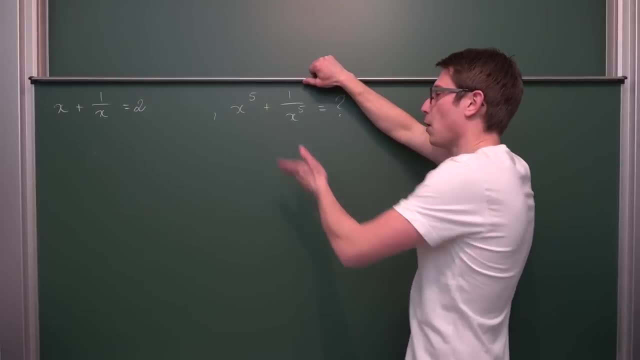 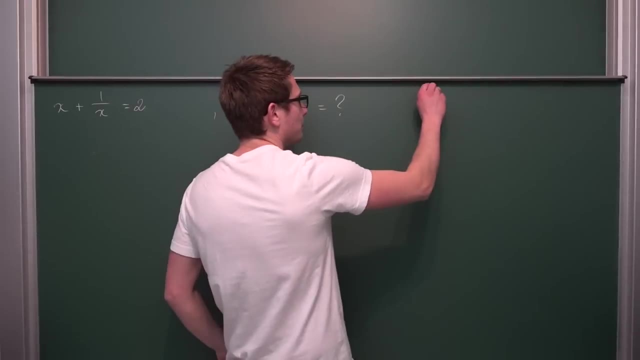 How could you go about finding out what x to the fifth power plus one over x to the fifth power is? At first, I would like to take a look at exponents in general. If you have something a to the n plus mth power. 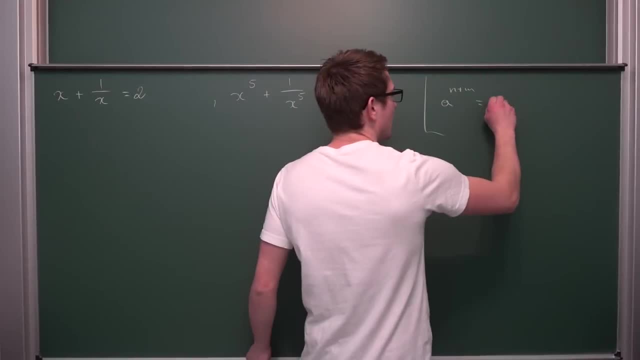 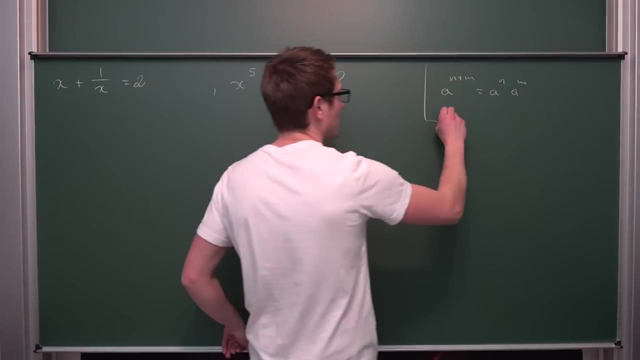 By the exponentiation rules, you can break this up into a to the nth power times a to the mth power, Meaning: okay, just to keep the long story short, If you have x to the fifth power, what you can do is you can turn this into x to the, for example, 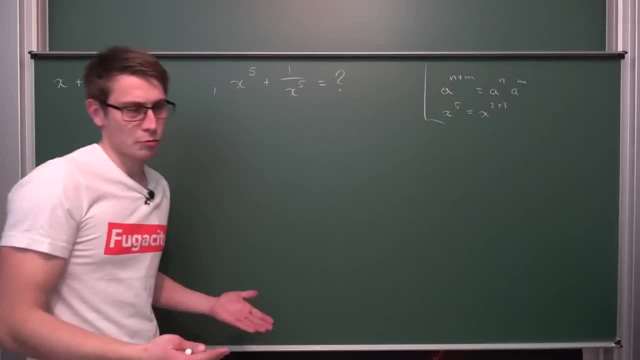 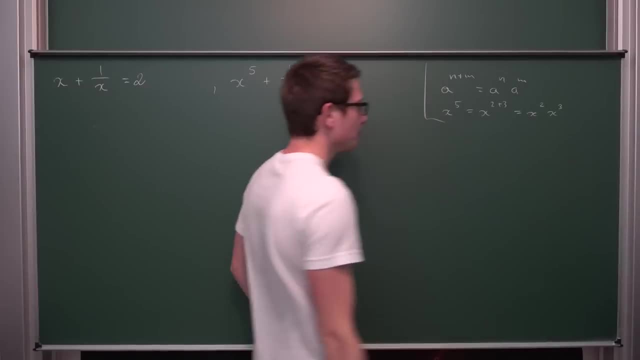 2 plus 3th power or 1 plus 4th power or the like, And then you can break this up into the multiplication of x squared times x cubed. Now this is going to help us later in the game, This tiny little thought here. 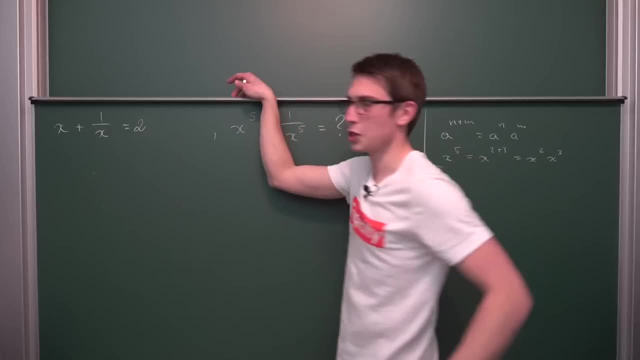 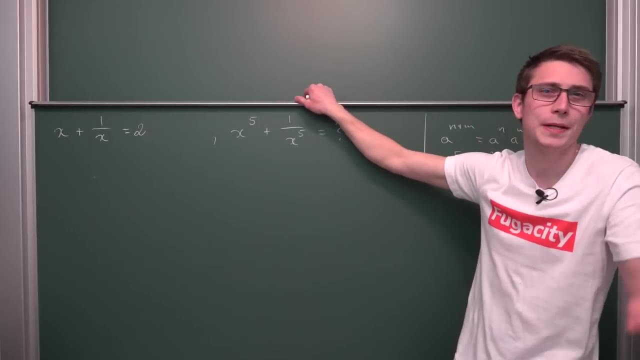 The first thing that we are going to do is we are going to square our original equation, Hence we are going to get some factor with x squared in it. We are going to repeat this process, basically up until we get to some kind of x to the fifth power. 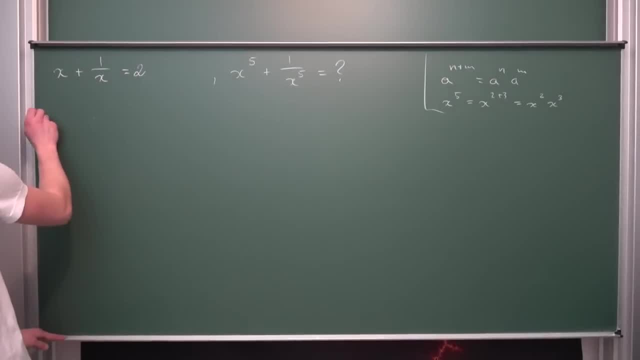 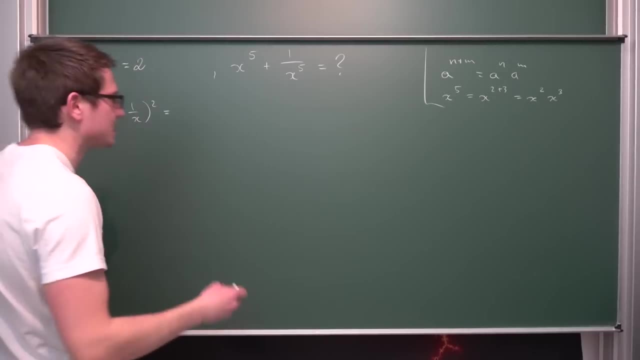 Now, if you were to square both sides of this first equation, We are going to get, on the left hand side, x plus 1 over x, But the whole thing squared is equal to 2 squared, which is nothing other than 4.. Now, what about the left hand side? 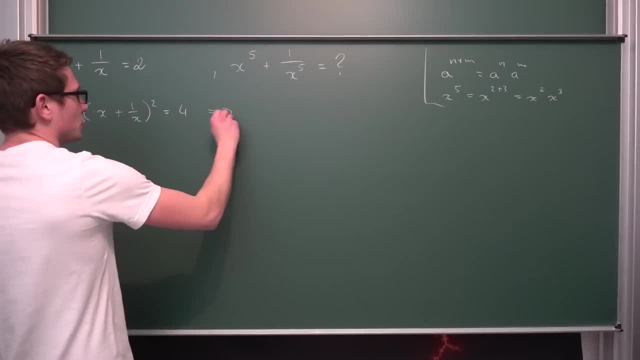 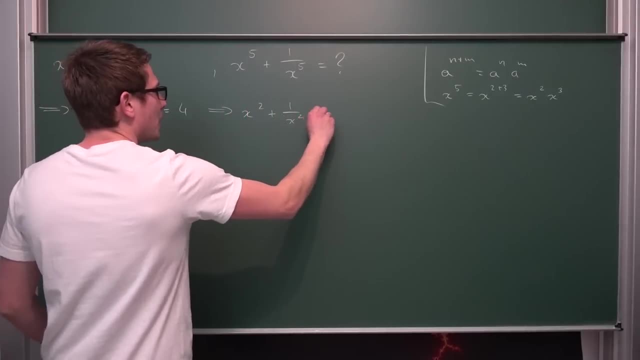 Well, this is just a binomial theorem, giving us overall- And this is where the magic is going to happen- basically. So this is going to give us x squared plus 1 over x squared plus 2 times the product of these two, So 2 times x times 1 over x. 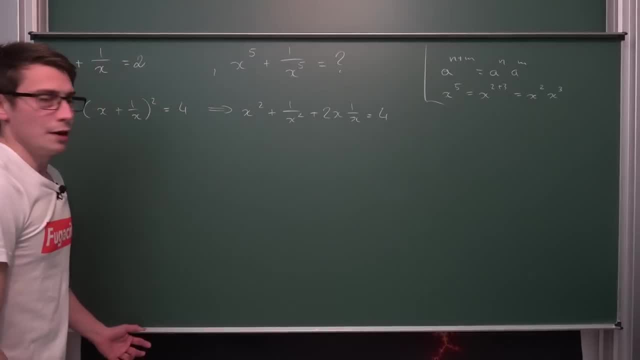 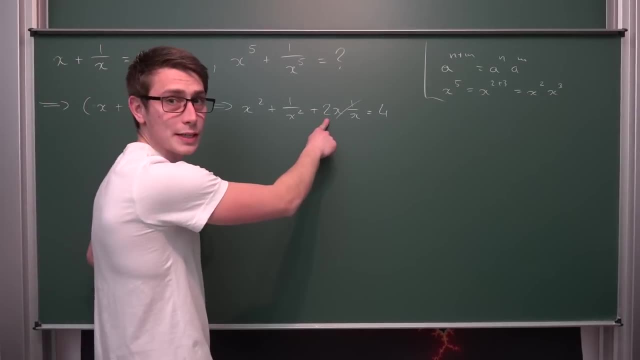 And all of this is still equal to 4.. Now, cool thing is: x times 1 over x. Well, this is going to cancel out. just giving us 2 here. Meaning this right here is a constant giving us something of the form x squared plus 1 over x squared. 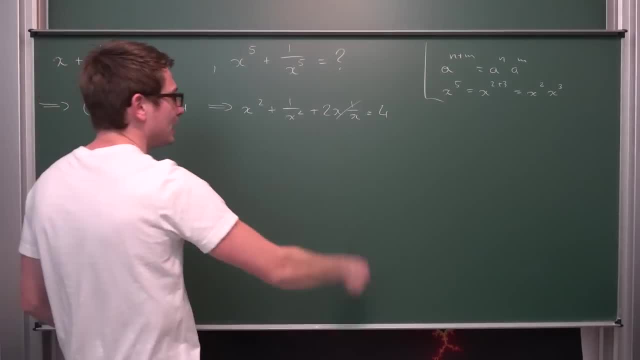 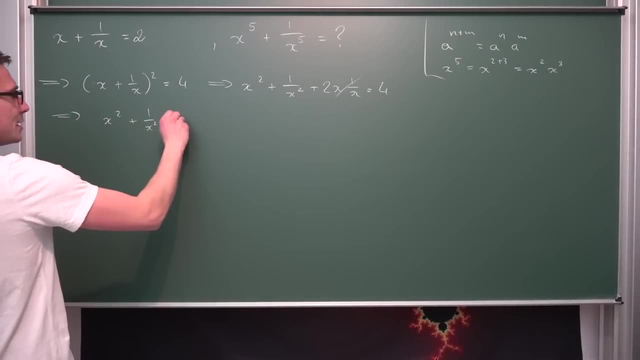 We are getting closer to x to the fifth power, plus 1 over x to the fifth power. Let us subtract 2 on both sides, Giving us that x squared plus 1 over x squared is nothing other than 2.. Okay, Same value as the original equation. 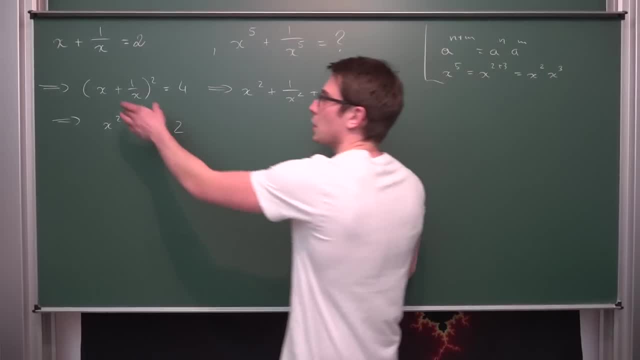 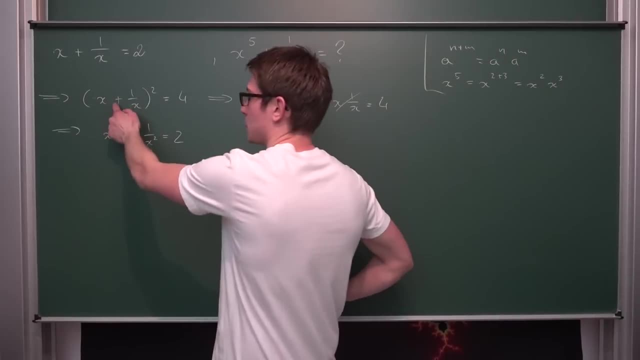 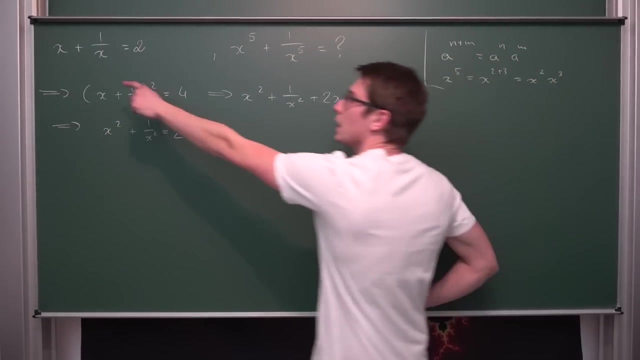 Let us continue with this thought. If you have our original equation squared basically, especially the left hand side, This is just multiplying x plus 1 over x with itself. So why not multiply x squared plus 1 over x, squared with x plus 1 over x? 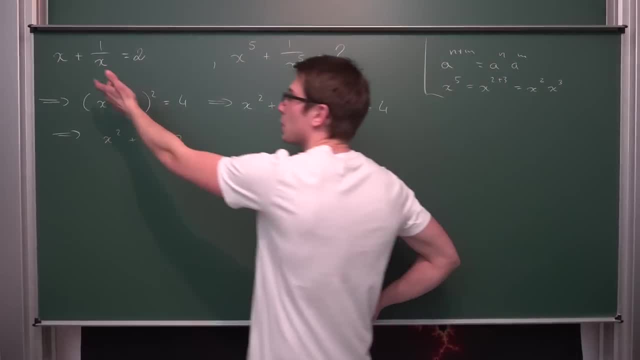 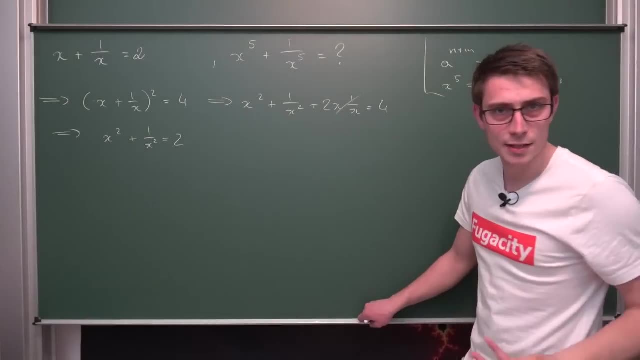 And then let's see what is going to happen. Since we know what x plus 1 over x is, This is nothing other than 2.. So we know the value of this, And also maybe this, This cancellation madness, is going to once again pop up in the process. 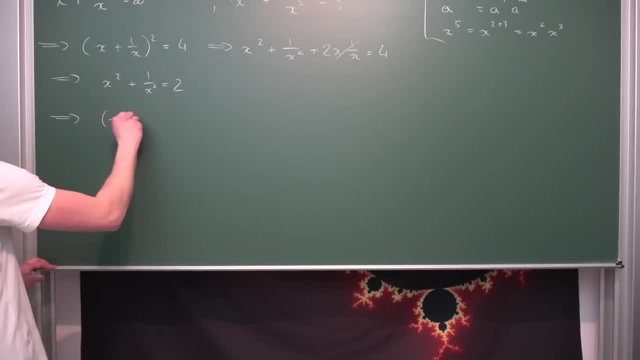 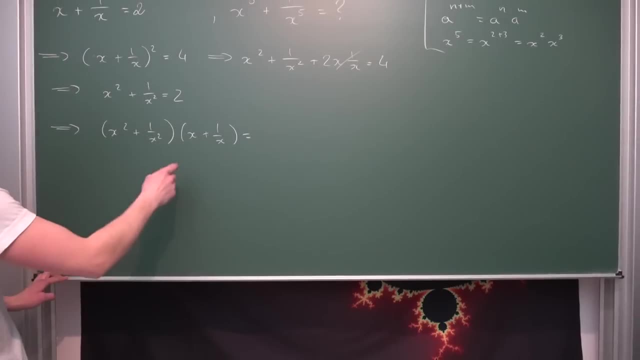 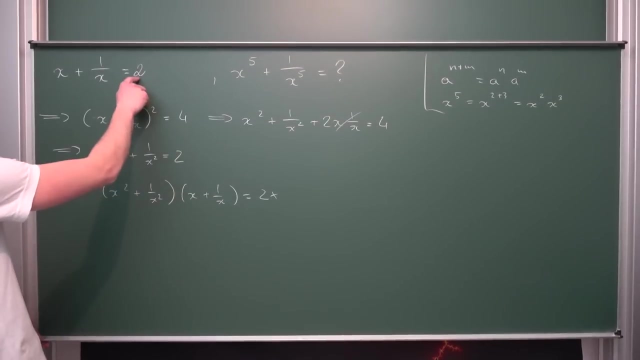 So what about multiplying x squared plus 1 over x, squared with x plus 1 over x? Well, if we take a look, So 2 was the value of x squared plus 1 over x squared times, And the value of x plus 1 over x is equal to 2 once again. 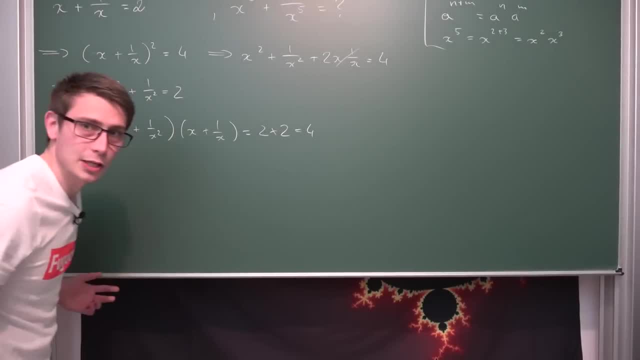 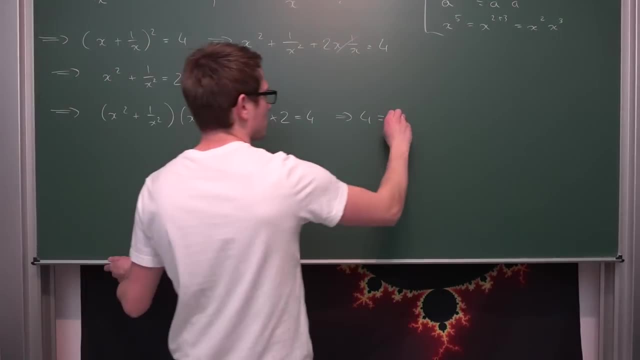 So this is going to give us 4 in the process. Now what about the left hand side? We are just going to multiply everything out. It is as easy as this. So 4 is hence equal to x times x. squared is going to give us x cubed. 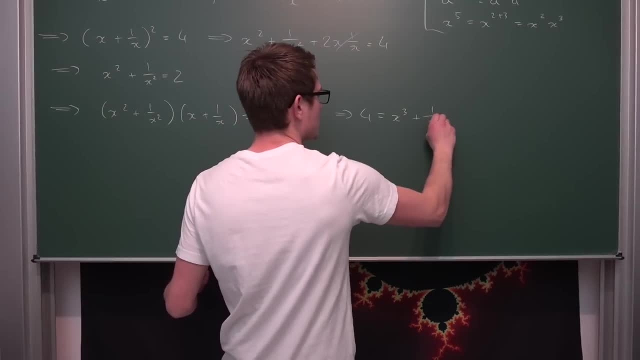 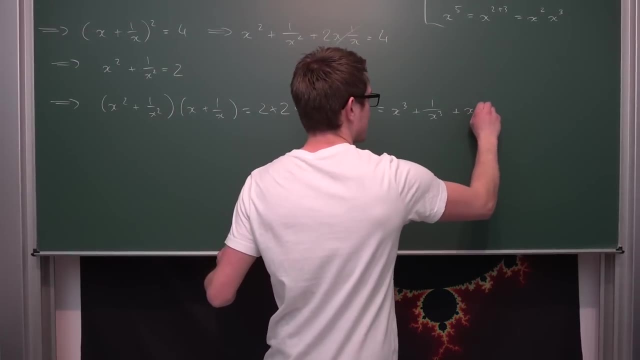 Same thing with the 1 over x parts, giving us plus 1 over x to the third power. Now, then, we are going to get x times 1 over x squared, So plus x times 1 over x squared, And also the other way around. 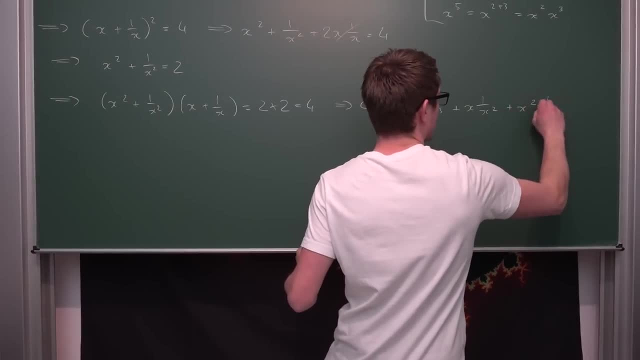 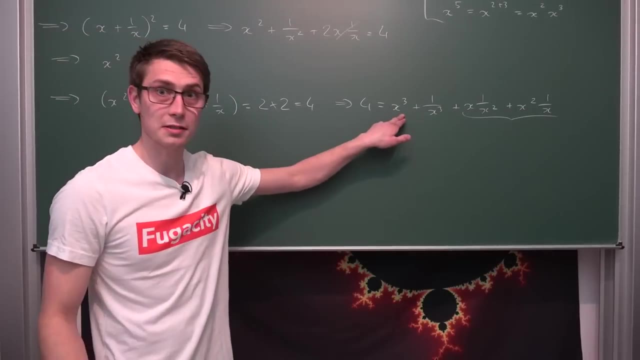 1 over x times x squared Plus x squared times 1 over x. Now, if we take a look at this, The last part here. So this first part is very, very good. This is something of the form x cubed plus 1 over x cubed. 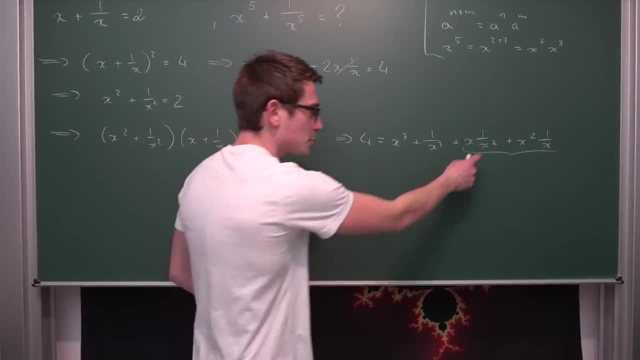 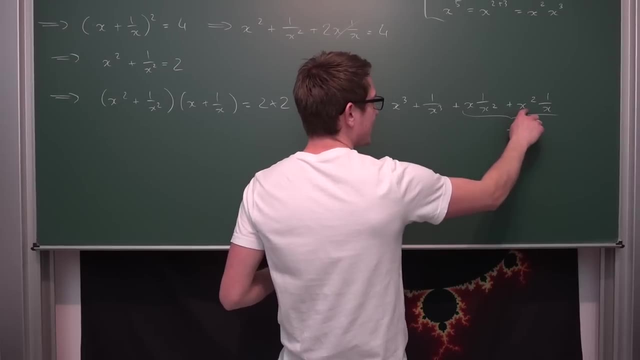 So we are getting even closer to what we have up here. But this part right here, This is actually pretty fabulous: x times 1 over x squared is going to give us 1 over x. And here, x squared times 1 over x is going to give us just x. 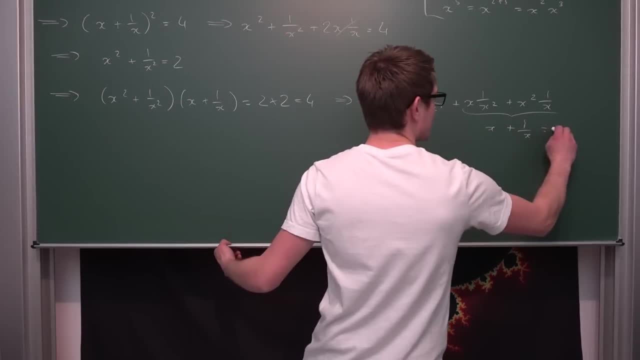 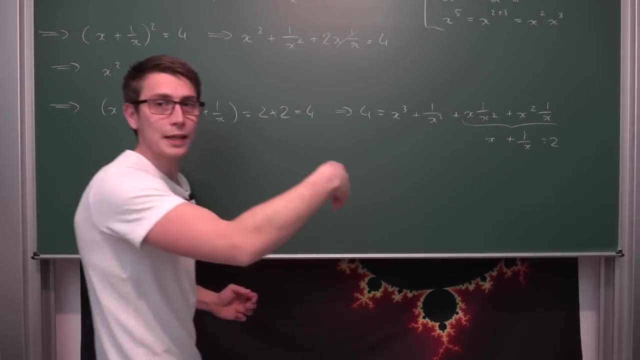 Oh, x plus 1 over x. We know what this is. This is equal to 2.. Meaning we have now the equation: 4 is equal to x cubed plus 1 over x cubed Plus 2.. Meaning if we were to subtract 2 on both sides. 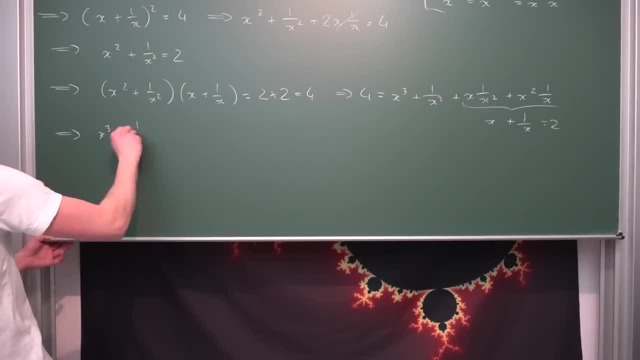 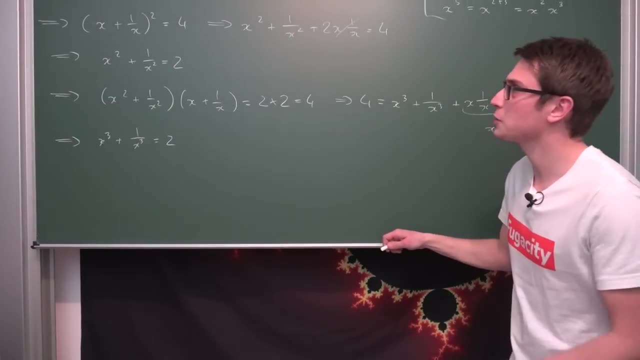 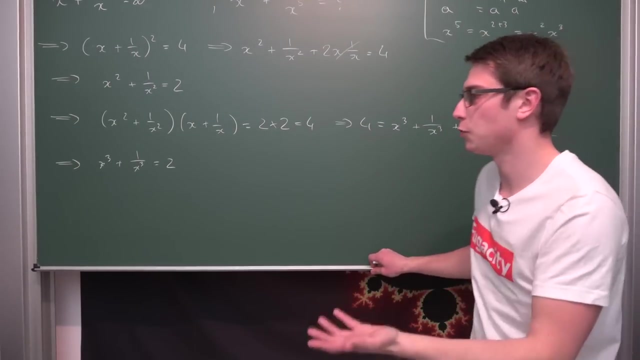 We are going to get that x cubed plus 1 over x cubed Is actually equal to 2.. Okay, Now we could continue this process, multiplying x plus 1 over x To the whole thing two more times, And then we are going to just solve for this part right here with the exponents. 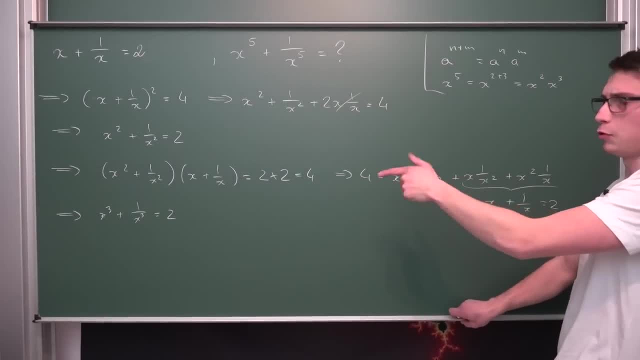 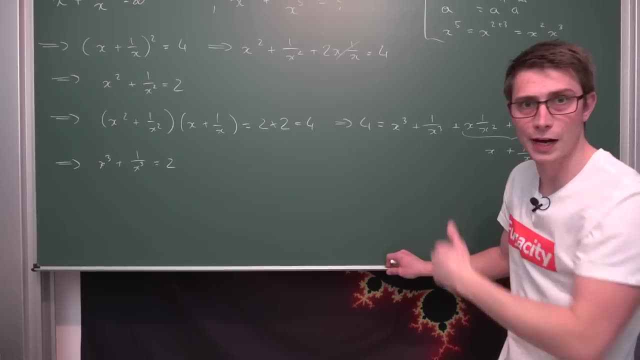 But by following our original thought. What we could also do is we could multiply these two equations together, Giving us x to the fifth power And, by this logic, also 1 over x to the fifth power in the process. So let us do this. 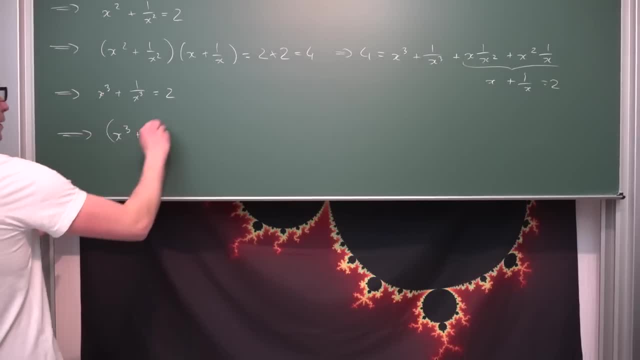 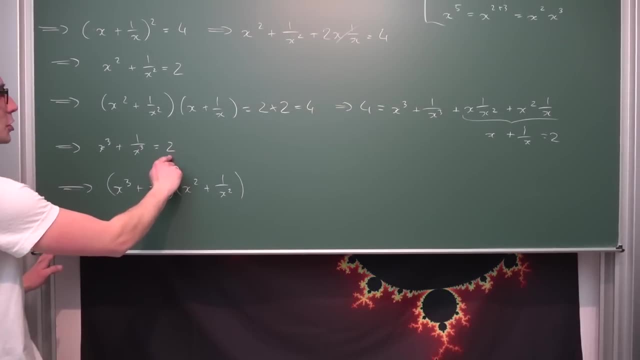 So what about x cubed plus 1 over x cubed Times? x squared plus 1 over x squared multiplied together? So we know what the values of these are individually: 2 and 2.. So meaning 2 times 2 is going to give us 4 overall. 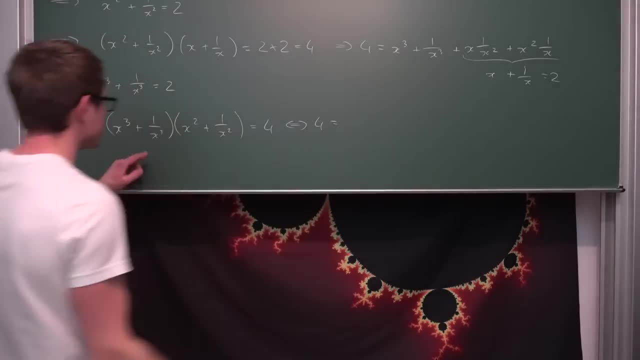 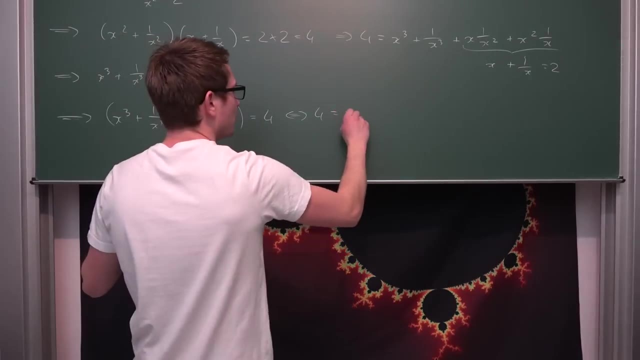 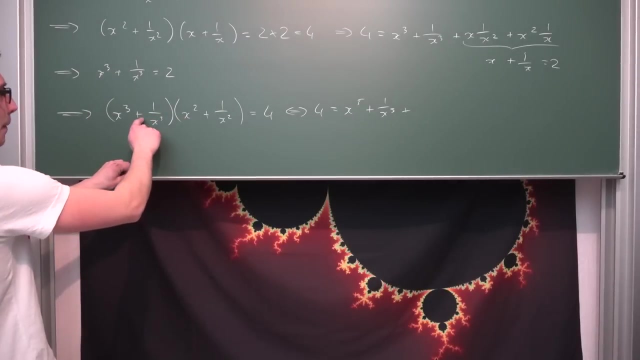 Now we can start multiplying everything out, Meaning 4 is equal to. Now we are going to get, just like here: x to the fifth power plus 1 over x to the fifth power. And also, what else are we going to get? x squared times 1 over x cubed. 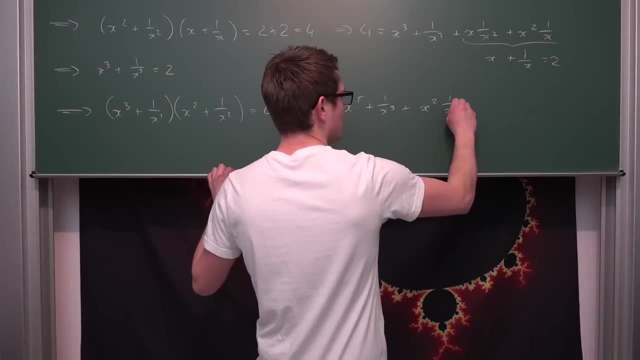 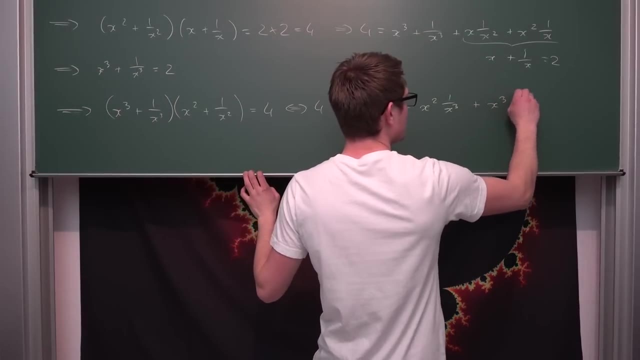 x squared times 1 over x cubed. Oh, we know what this is. This is going to give us 1 over x. Let me take a wild guess here. Next sum is going to be x cubed times 1 over x squared. 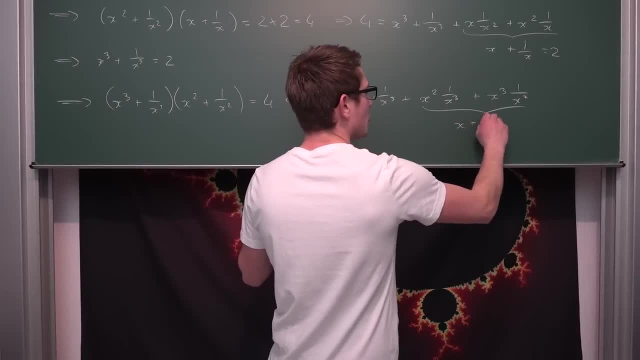 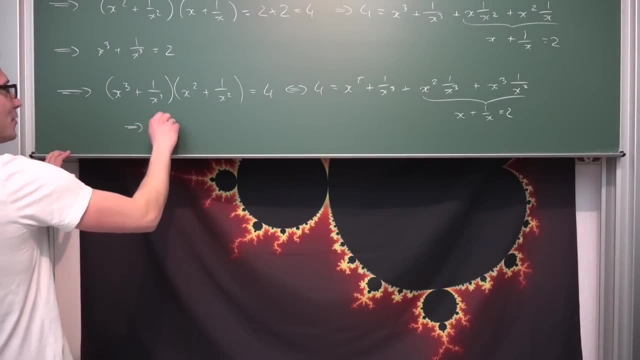 Meaning: what we are going to get here once again Is x plus 1 over x. But we know what this is. This is nothing other than 2.. Meaning: by subtracting 2 on both sides, We are going to get the very, very boring solution to this problem. 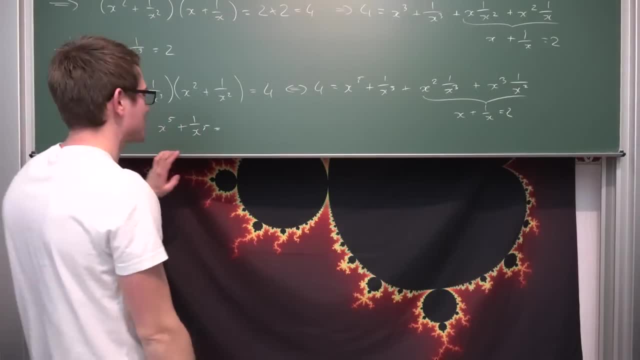 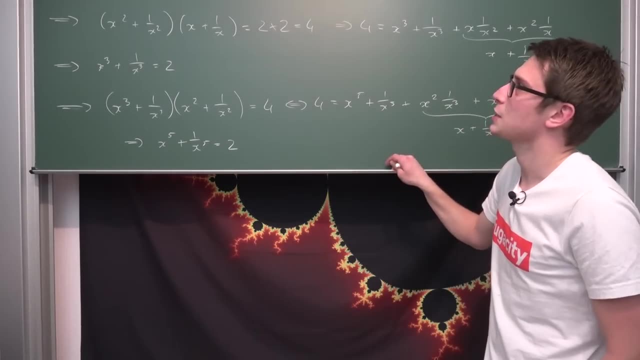 That x to the fifth power plus 1 over x to the fifth power Is actually equal to 2.. Now the cool thing about this is that This is actually some kind of fixed point you could say For all of these powers that you are going to get here. 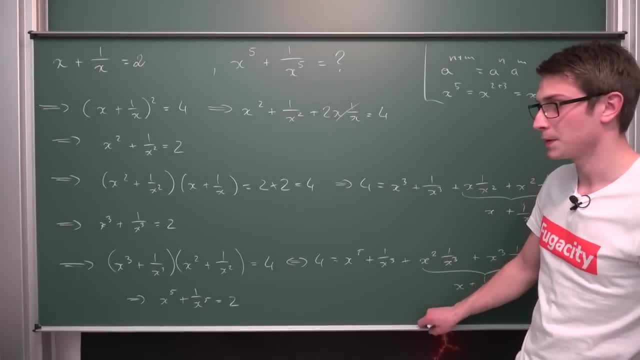 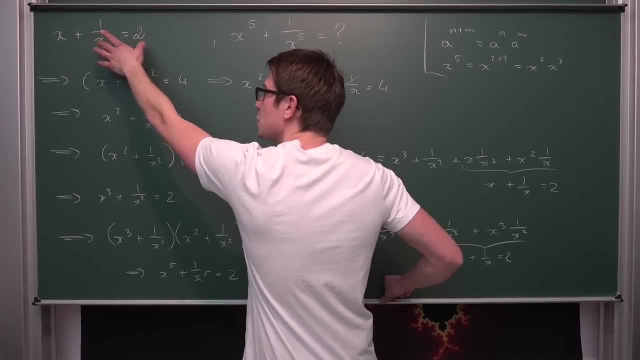 You can probably show this by induction. You are going to get that This is going to be equal to 2. At least if we start with our original equation being equal to 2. We can actually just set this equation equal to n. 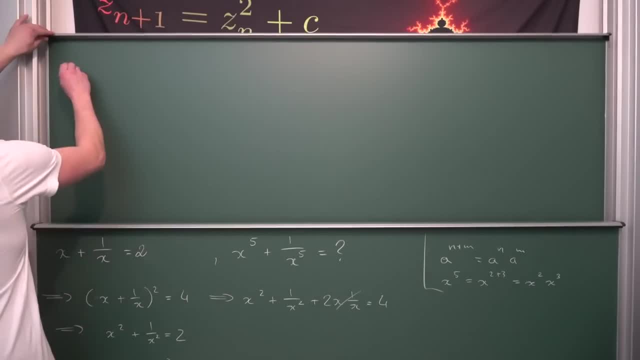 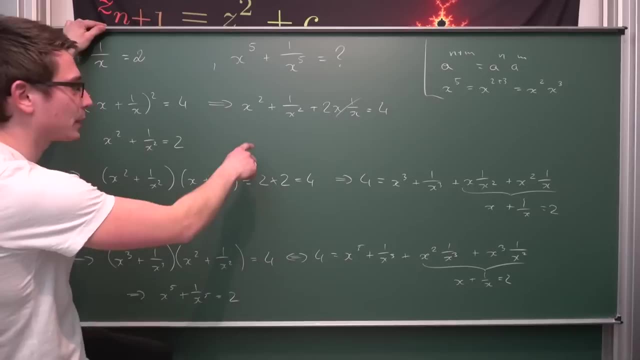 And then we are going to see what happens. Okay, So if we have x plus 1 over x, Being equal to n, Now what about our squaring? Okay, If we were to now square this, Not much is going to change in the logic. 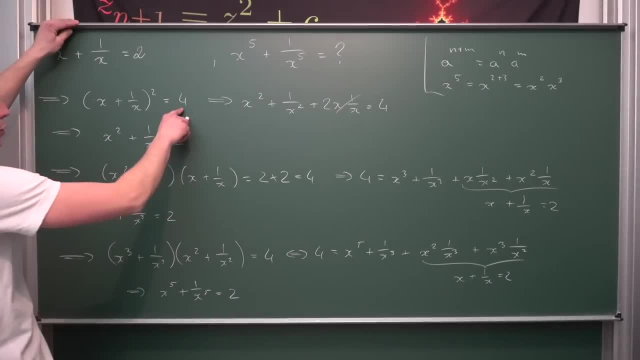 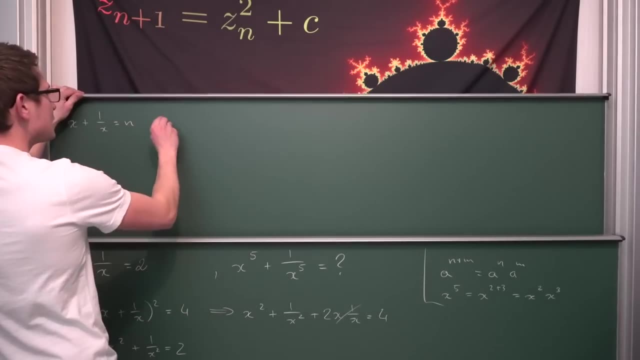 Except for: Okay, Our 2 was squared here To 4, meaning we are going to get n squared And then we are going to subtract 2 from this whole thing. So we are going to get By just solving everything once again. 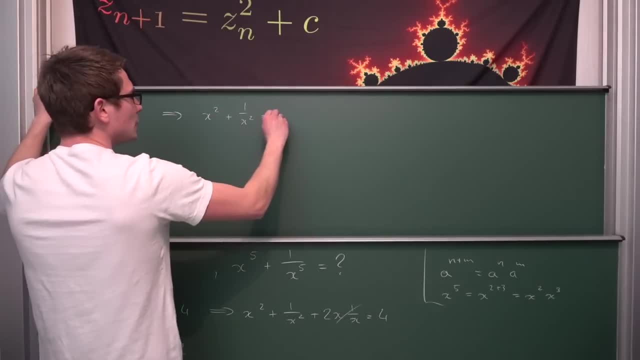 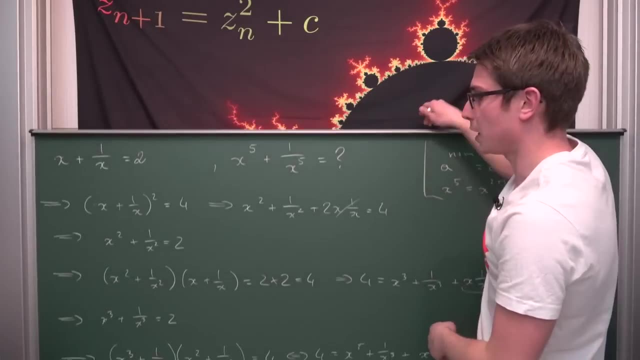 That x squared plus 1 over x squared Is equal to n squared minus 2.. And now we can continue with this process. What else have we find out Now if you were to multiply our x squared plus 1 over x squared? 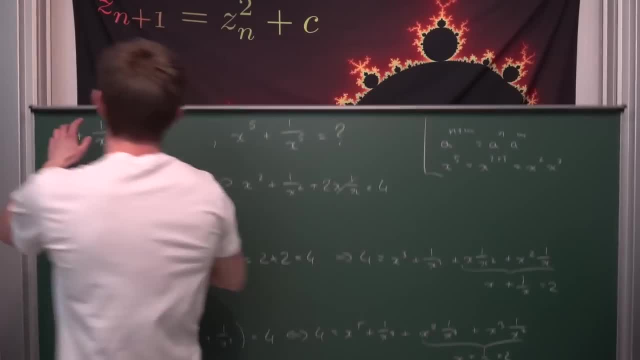 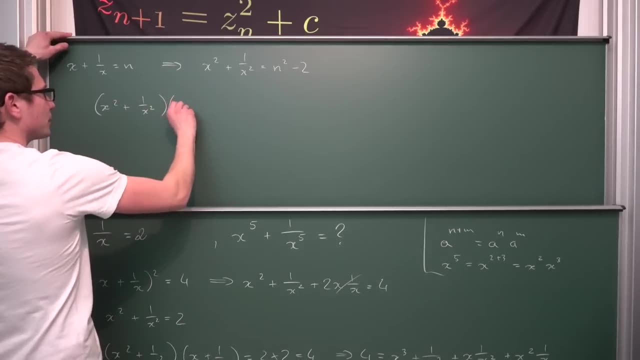 With x plus 1 over x, This next thing that we are going to do. So x squared plus 1 over x. squared Times, x plus 1 over x. We know that this, right here, is nothing other than n By the original equation. 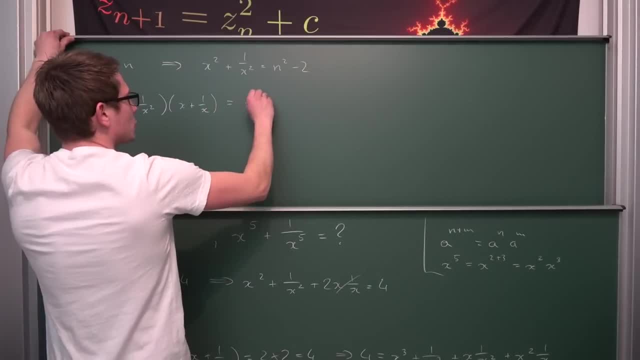 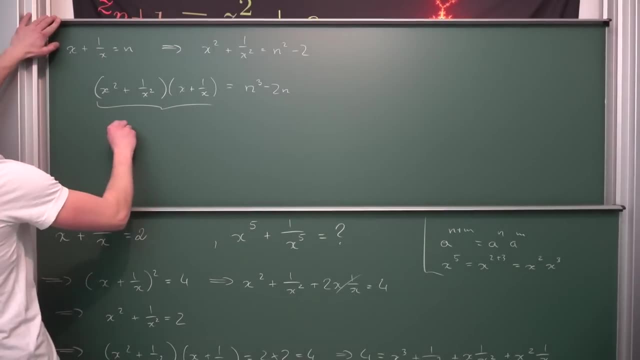 Meaning also this right here is n squared minus 2.. We are going to get n to the third power minus 2n, And if we were to multiply everything out, We know that this right here is going to result in x cubed. 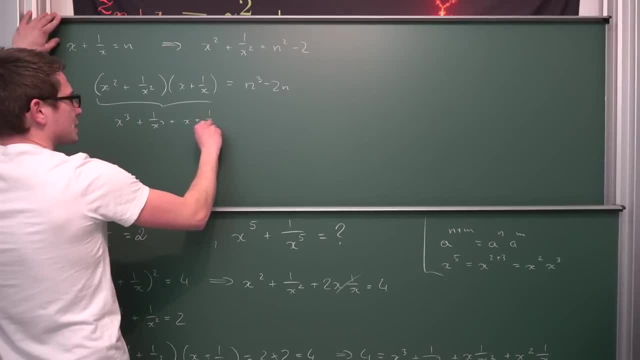 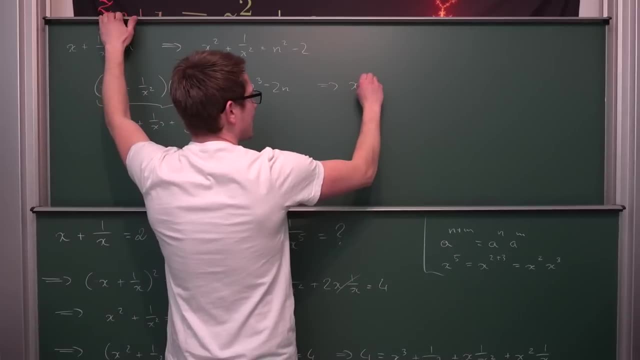 Plus 1 over x cubed. Plus x plus 1 over x. But this right here is nothing other than n Meaning. if we were to subtract one more n on both sides, We are going to get that x cubed Plus 1 over x cubed. 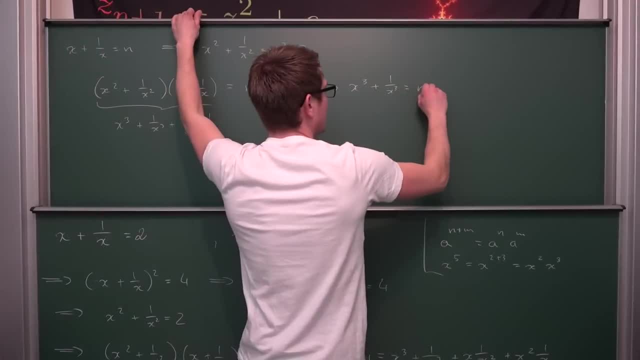 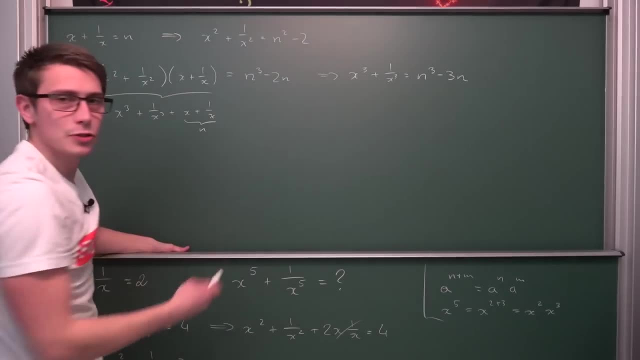 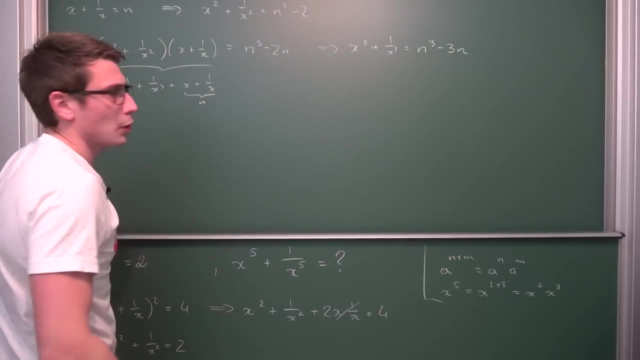 Is actually nothing other than n to the third power minus 3n. And well, Now we can just multiply these two together To get our final equation, basically, Or our final solution, Just in a generalized fashion, What we also find out. 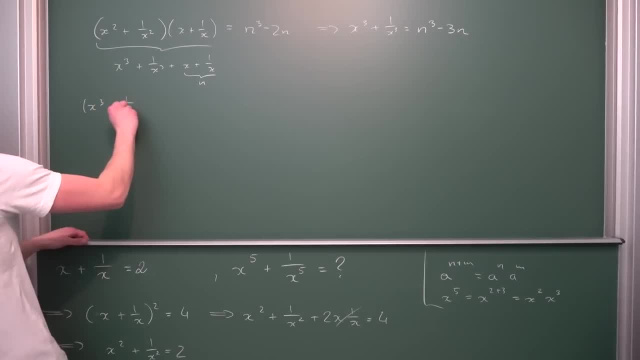 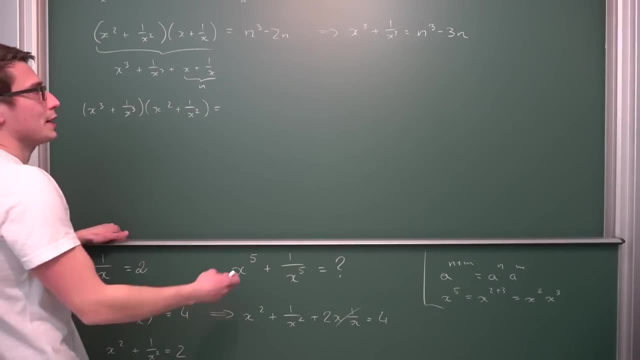 Or found out before Is that if we multiply x cubed plus 1 over x cubed With x squared plus 1 over x squared, What we are going to get is, on the one hand, The multiplication of these two, obviously, So we are going to get n squared minus 2.. 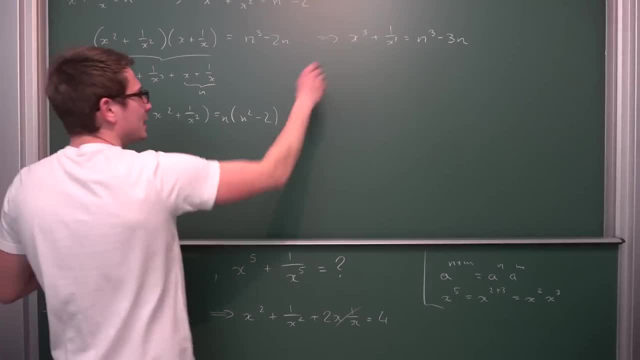 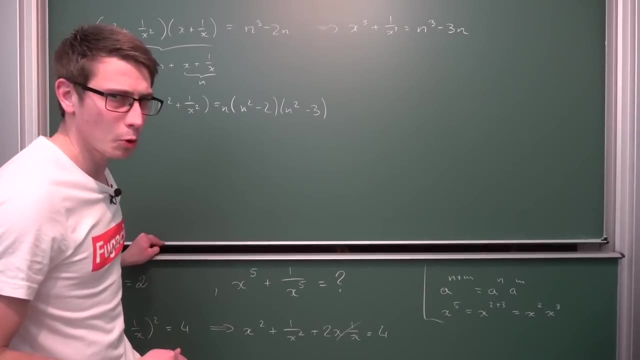 And this thing: right here We can factor out a common factor of n, So n times, Then we are going to get n squared minus 3.. So here is a nice pattern that is going to pop up, And you can probably generalize this even more. 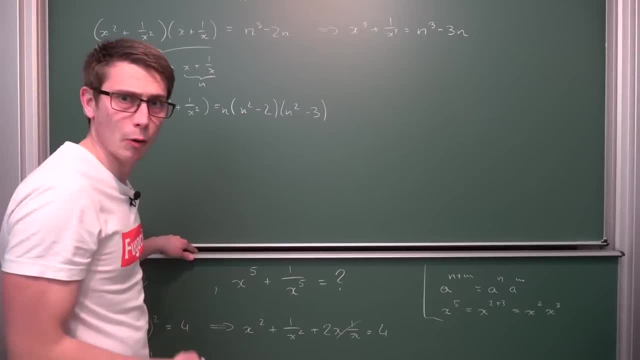 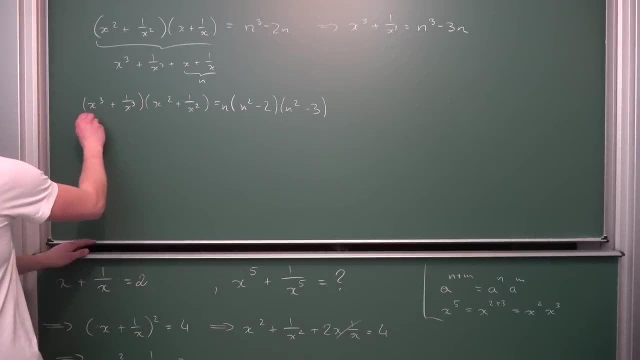 To some arbitrary power Instead of x to the fifth power Plus 1 over x to the fifth power. I leave this up to you To solve as an exercise to the viewer, And we also know what this right here is going to weigh. 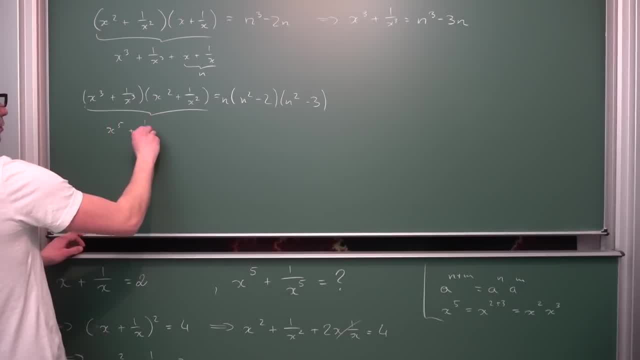 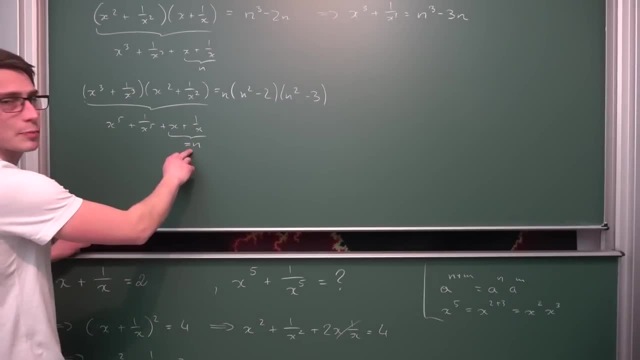 I too name the x to the fifth power Plus 1 over x to the fifth power Plus x plus 1 over x, And we know that this, right here is once again equal to n. So if we were to subtract n on both sides, 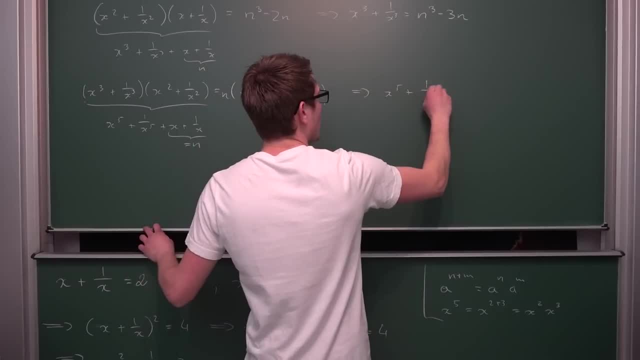 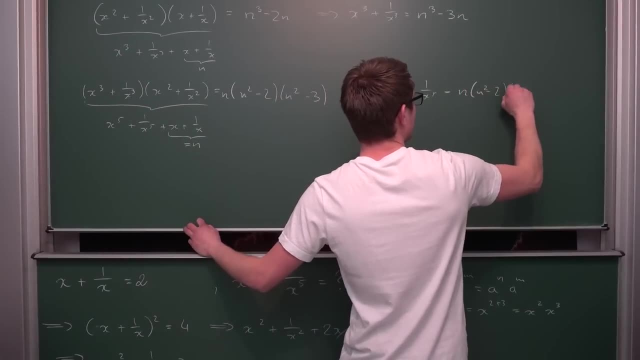 We are going to get that x to the fifth power Plus 1 over. x to the fifth power Is n times n squared minus 2.. Times n squared minus 3. Minus n. But we have n as a common factor. 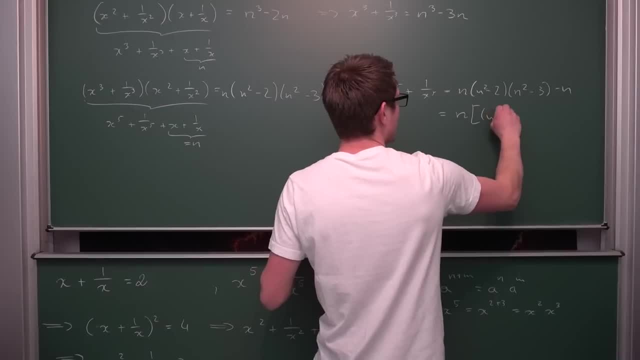 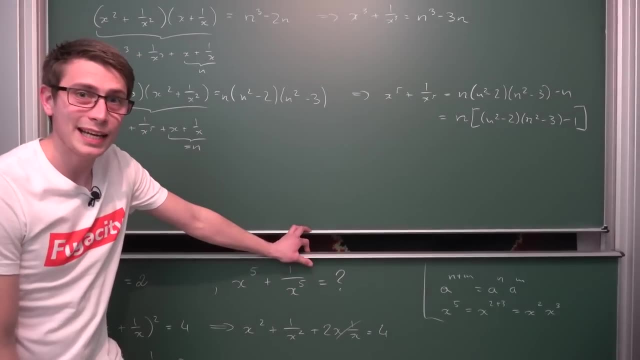 So the final formula in a generalized fashion Is: n times n squared minus 2.. Times n squared minus 3. Minus 1.. Now you can plug any all initial value in And see if you can find out the solution. 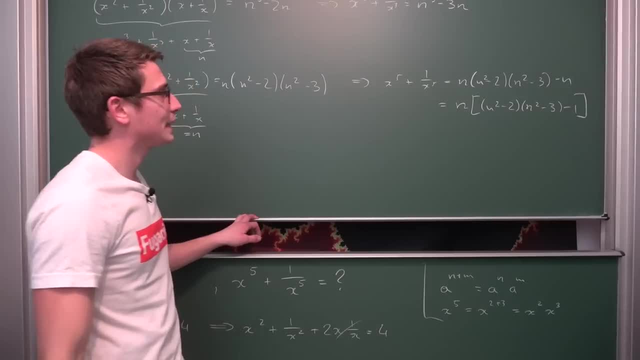 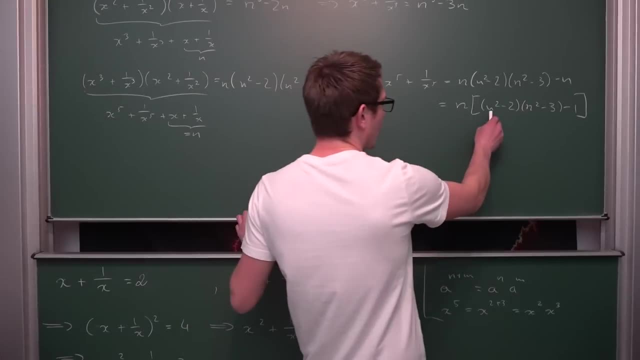 By doing a bit of calculation. For example, What about n being equal to 1.. What is going to happen here? I am actually wondering. If you plug in 1. We are going to get For n equal to 1.. 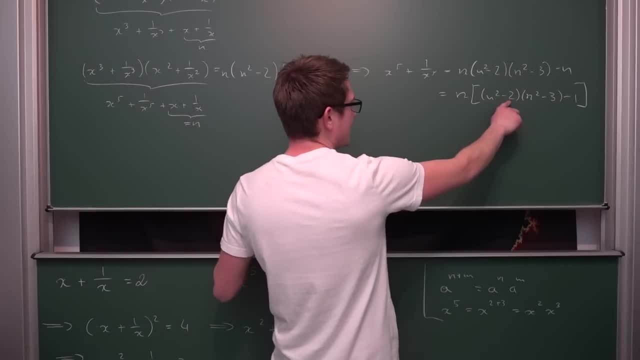 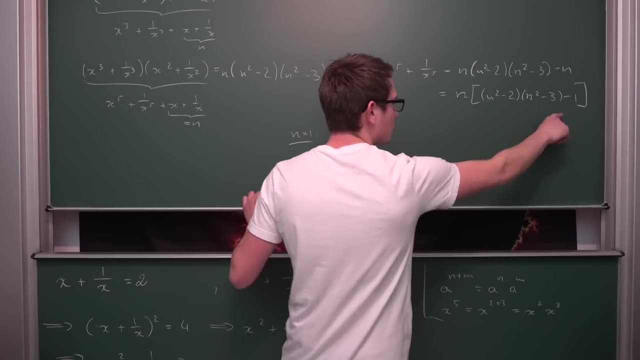 We are going to get 1.. Minus 2 is negative 1. Then we are going to get negative 2. So this is positive 2. Minus 1 is 1.. 1 times 1 is 1.. 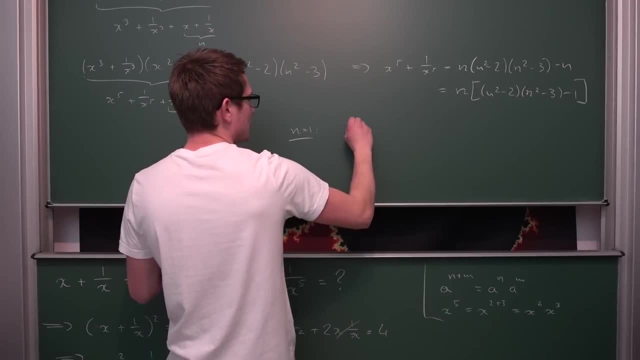 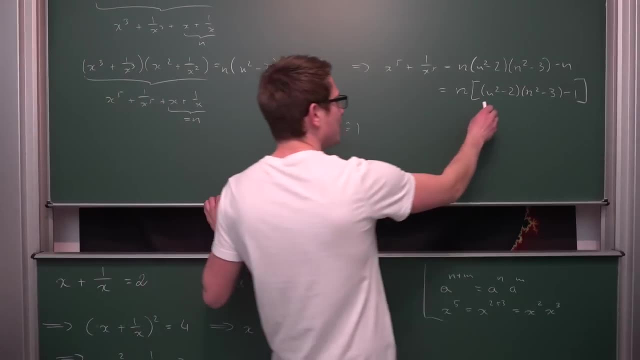 Okay, we are going to get That. this right here is going to be equal to 1.. Now, what about n being equal to 3.? Okay, I haven't tried out any values, So let's just see n being equal to 3.. 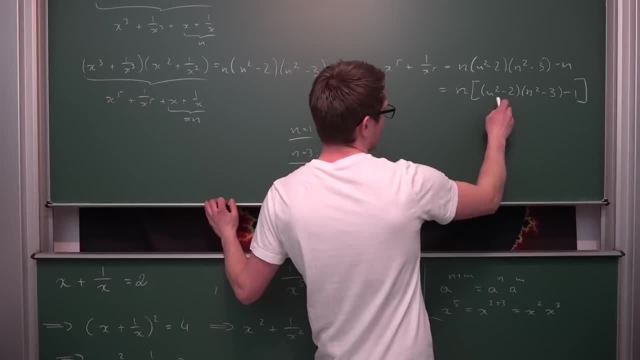 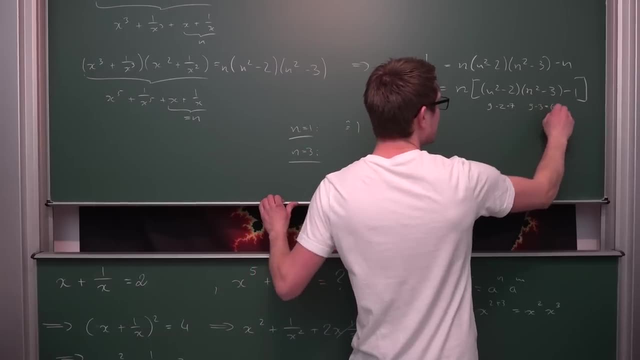 So this right here is going to give us 9 minus 2. Is 7.. Then we are going to get 9 minus 3 is 6.. So this right here is going to give us The meaning of life. 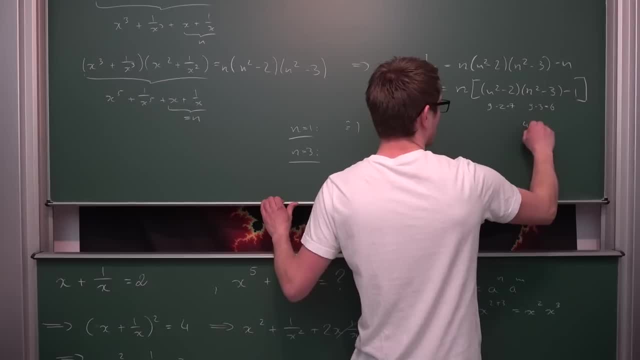 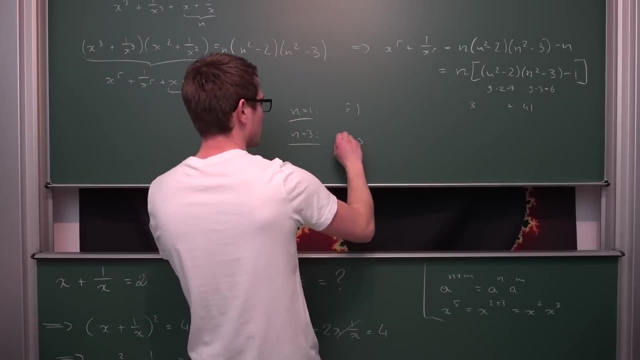 42 minus 1. Is going to give us 41. Times. and we said 3, right? Yeah, Meaning this is 123.. And 123 is not a prime number. It's divisible by 3.. Yeah, And so on and so forth. 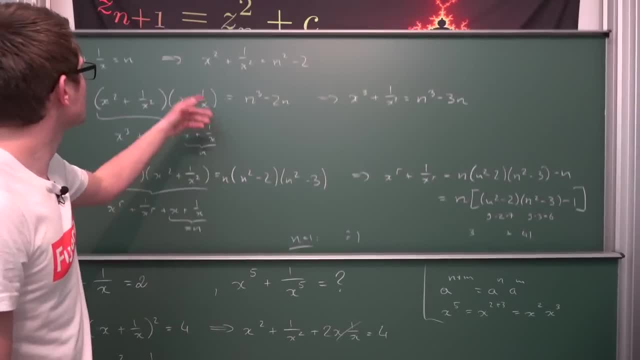 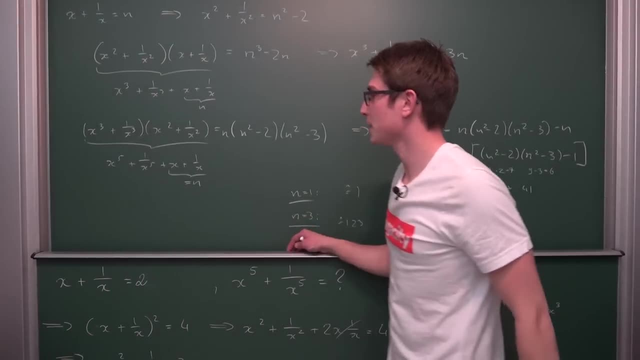 Try to find out a few values. You can also use fractional values, Obviously, Or square roots, Okay, As the starting value. Just try to play around with this formula A tiny little bit, And maybe you can find Even more of a generalization. 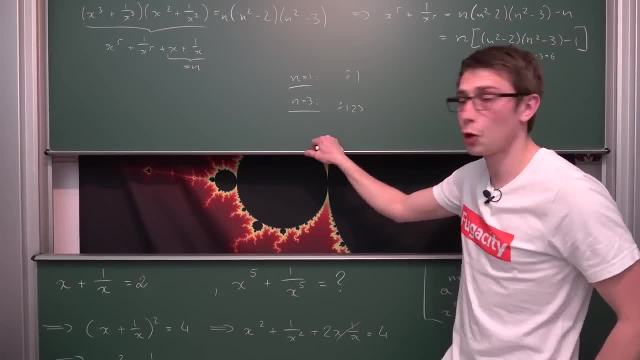 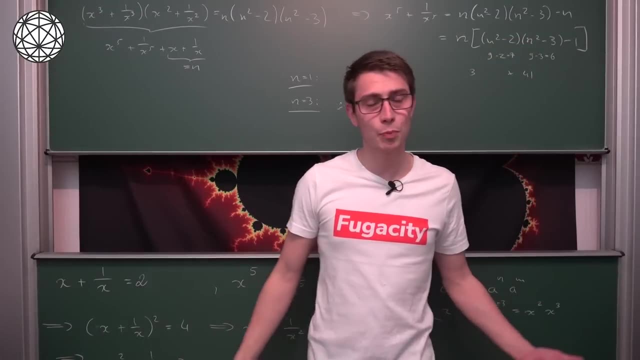 In the process, And this concludes today's video, And if you did enjoy what you have seen today, If you are interested in more algebra, Calculus And all of the like, Then I invite you To try out the contents Of today's sponsored brain. 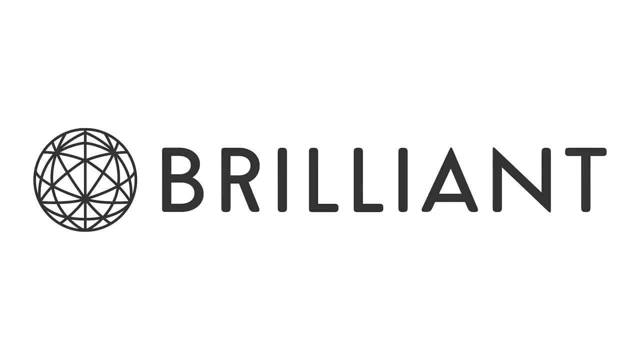 Who are kind enough to sponsor Yet another video Here on this channel. Man, This problem was hella refreshing. I really liked this one. I don't know why It was easy. The answer was kind of obvious Even after the first iteration. 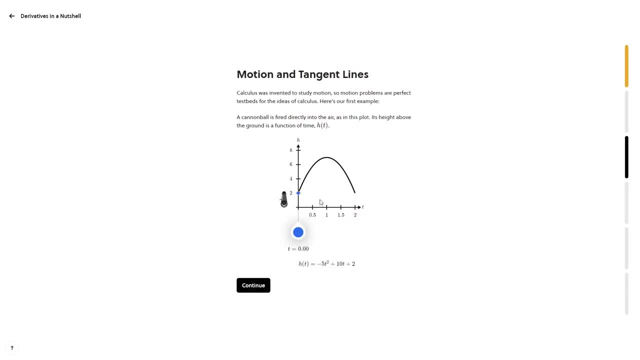 But it was still fun To solve through it. And if you are a sucker For solving Edge break equation And maybe you also want to see The intuitive nature Behind all of these equations, Especially polynomials And their graphs. 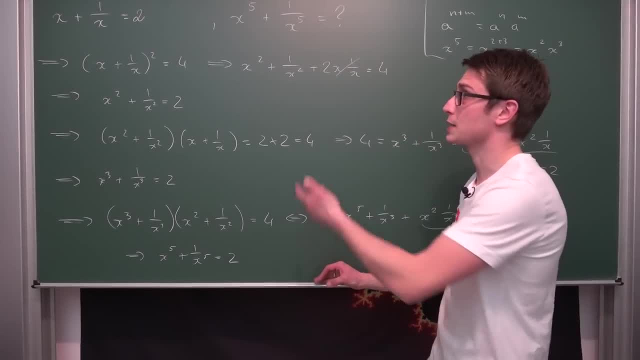 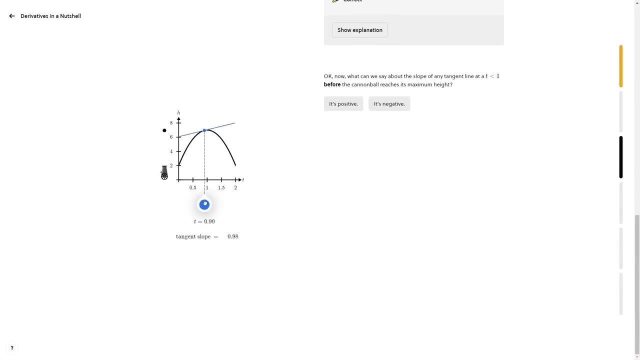 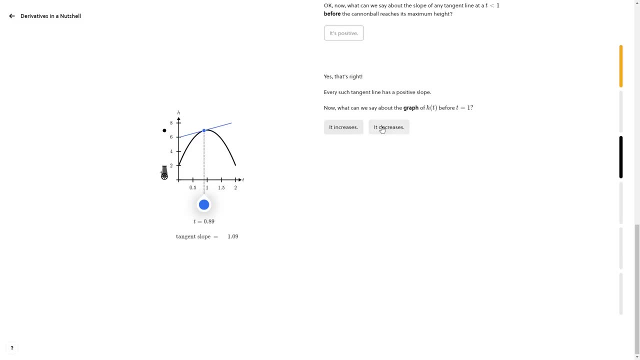 Pre-End Is an online learning platform And app With over 60 interactive courses In all topics, Be it mathematics, Physics, Chemistry- No matter what it is You are seeking after, Pre-End definitely Got something up. 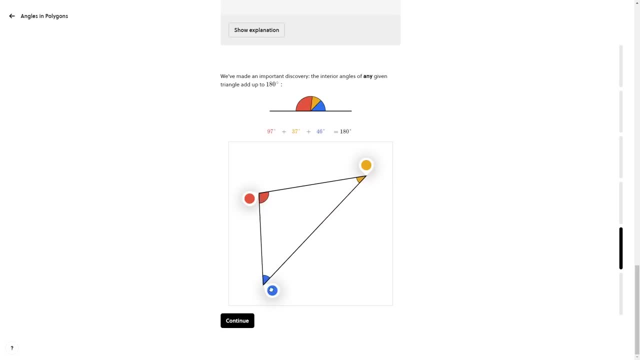 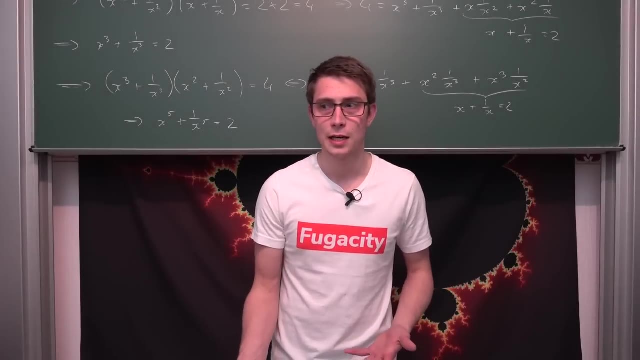 The sleeve For you, And if you are one of the people Who learns By taking a look At something Graphically, Which is going to give you An intuitive understanding Of the problems At hand, Then Pre-End. 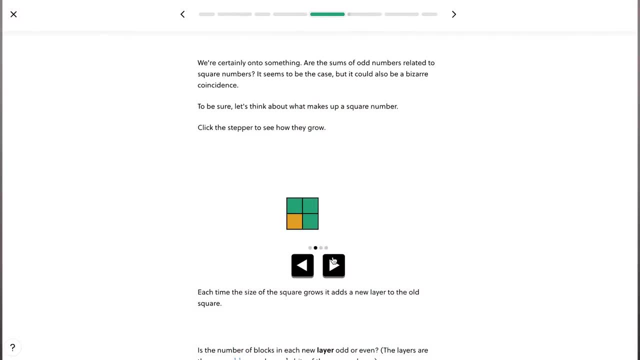 Is definitely a platform That you could be interested in. Interactive courses Means That you are going to have, For example, A parabola given, Or maybe An algebraic structure, Be it Just the multiplication Of two natural numbers.